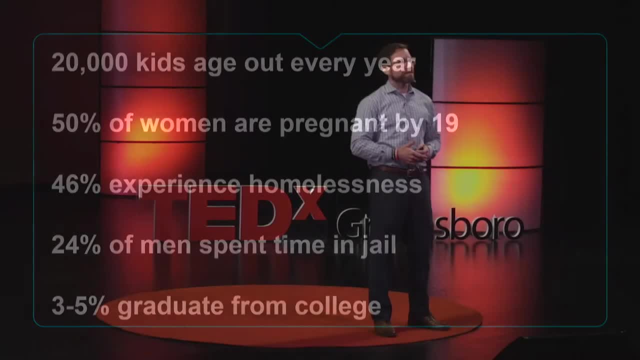 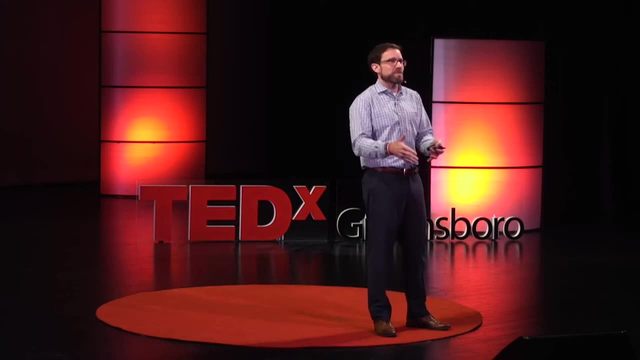 heartbreaking to watch this happen to these kids And I came to this crossroads really early in my career. Do I give up on this job for something less hopeless, less desperate, Or do I commit myself to trying to make the system better? And so I'm sitting in Cody's apartment one day and we're going through his independent living. 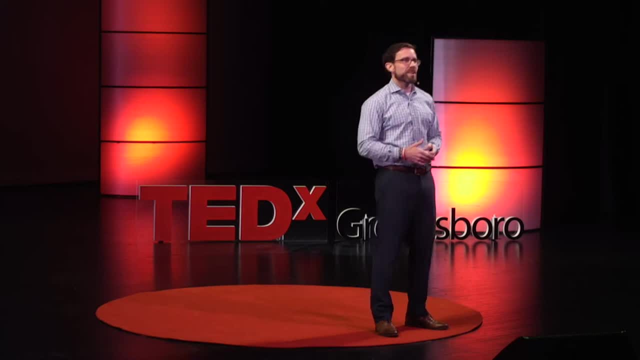 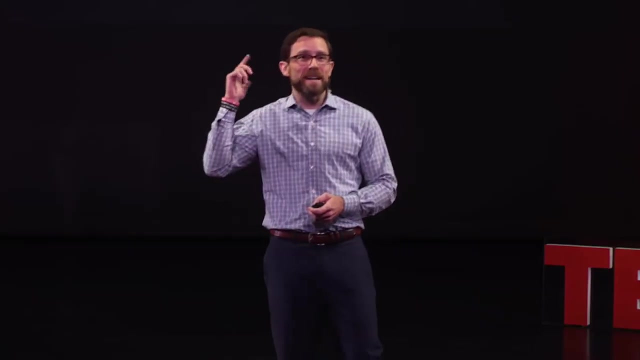 goals, the checklist. I'm doing my thing as this young social worker and, you know, Cody interrupts me abruptly And he says: do you know my story? And I said no, not really. And he said I think you need to know my story. And now, in the back of my mind, I'm thinking: 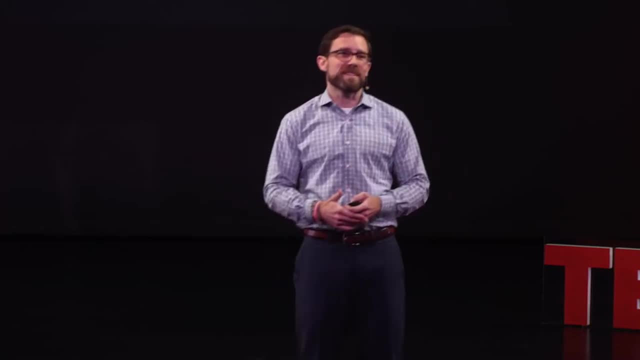 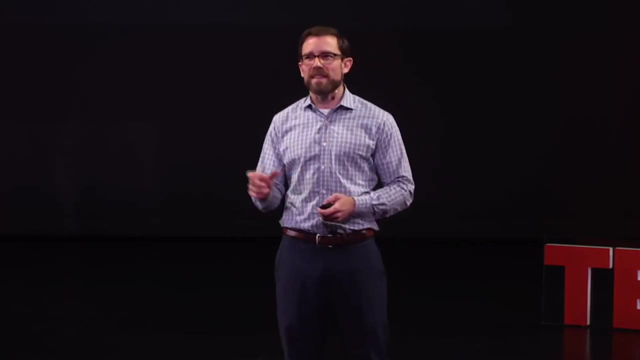 we don't have time for this right. Clock's ticking. you're going to age out. we need to get to it, Right. But I decide to listen And Cody starts by telling me that he was removed from his family on his 11th birthday And he describes that day for me, The social worker coming to. 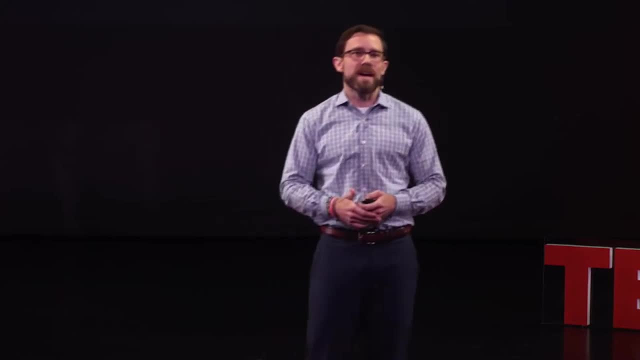 school, picking him up, taking him to his first foster family's house, Abruptly, immediately separating him from his mom, his siblings, everything, everyone He had ever known, placing him with a family he had never met before in his life. 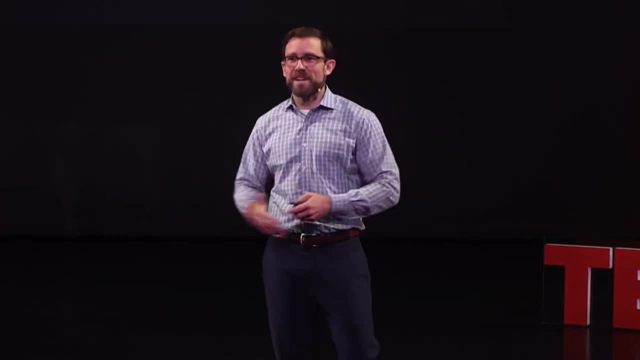 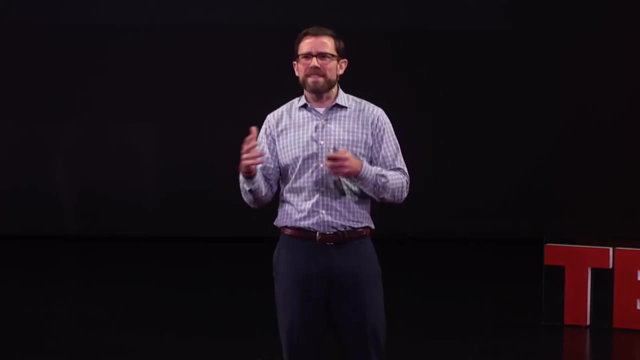 And so then he goes on to tell me about the next 17 different foster care placements that he's in, And he tells me about all the different people and you know, social workers and therapists and changing schools all the time and the stress, the confusion of all of it. And then he starts. 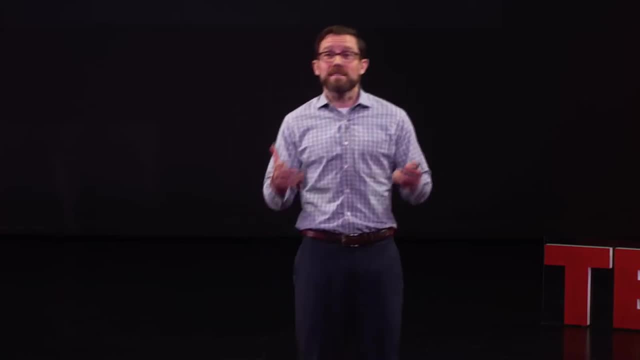 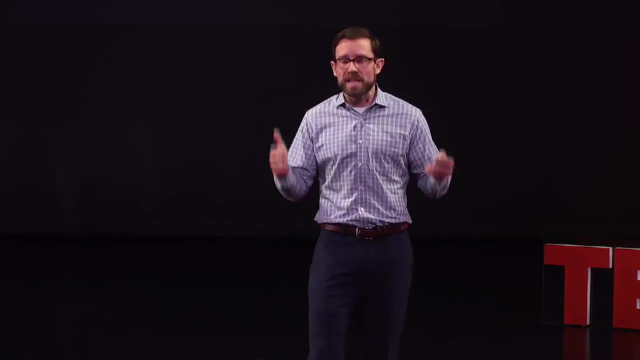 telling me about the fear, The fear that he had of turning 18, aging out being on his own. what's going to happen, Right? And so I start telling Cody this incredible story, but I don't know where in my life would. 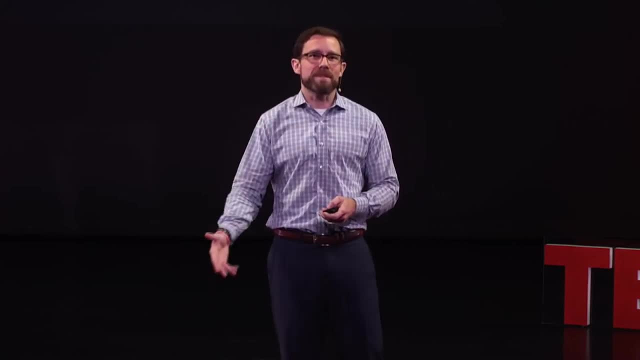 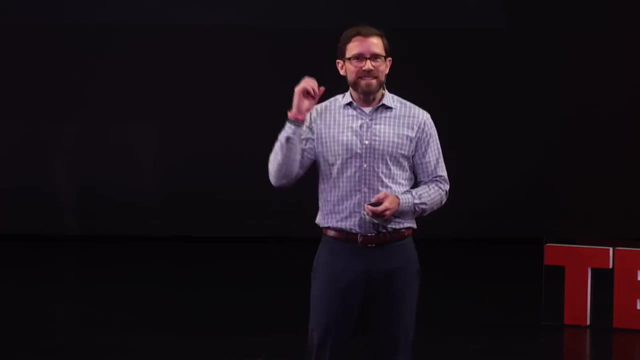 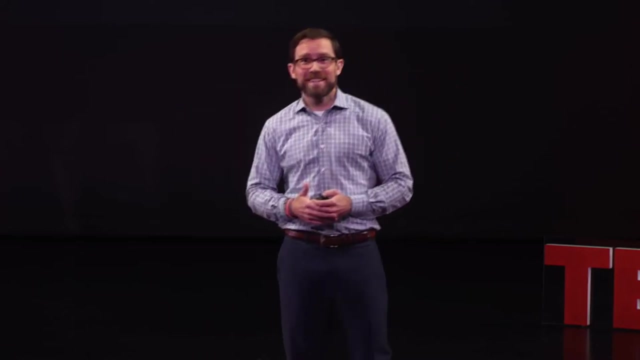 I be at this point And he starts saying spoilers. and I get up and I read this in a magazine: Victoryで squad. And I just thought why? And he got mad. I mean, like you're very sweet this time, Tell me all the reasons. I'm like I was too young to know that. Yeah Well, I was at the same age as Cody and we chose an opportunity when we found out our first family had toast, And this time I was um pretty sure, uh, this one is going to be away. 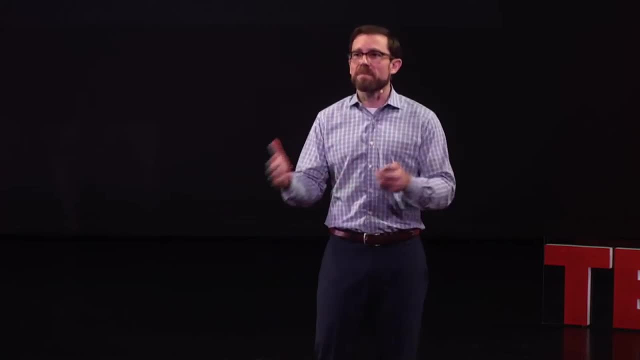 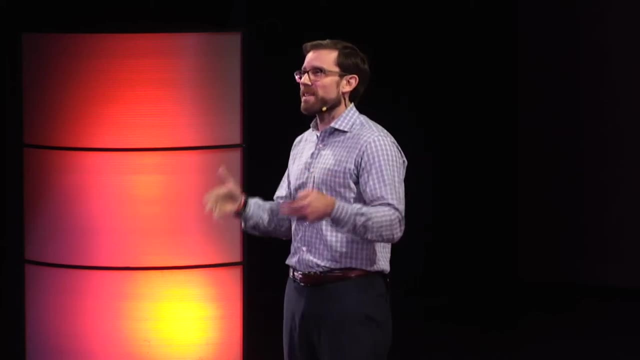 with us. No, Cody. we released a feature documentary film called from place to place and We followed three young adults for two and a half years post foster care to see what happens. We take this really deep dive into what life looks like for kids who age out. 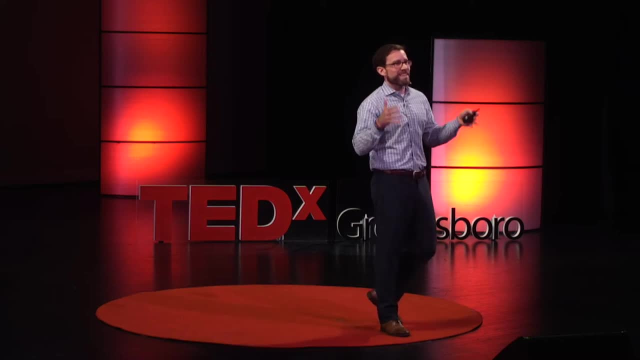 We see what happens when Kids are fully seen and heard by people in a position of power to make the system better, and the film goes on the screen all over the country and It has this impact on child welfare, training and education and practice and policy- All right, which I'll talk about. 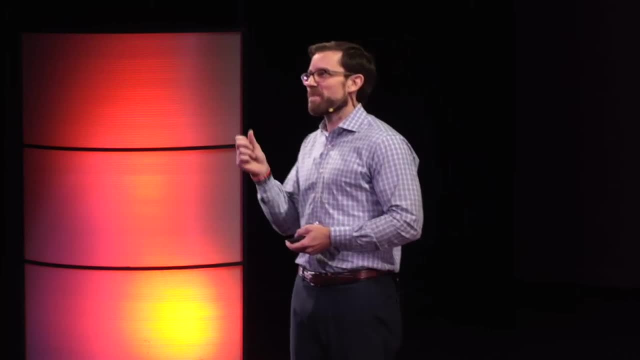 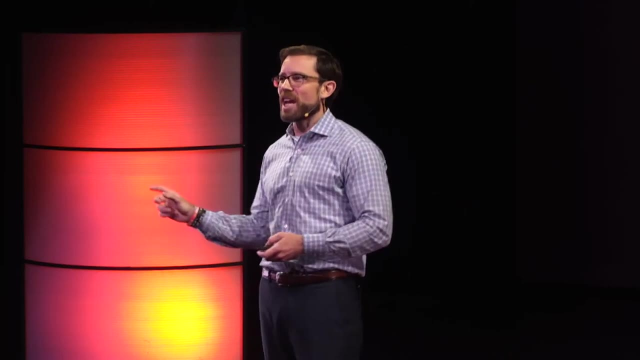 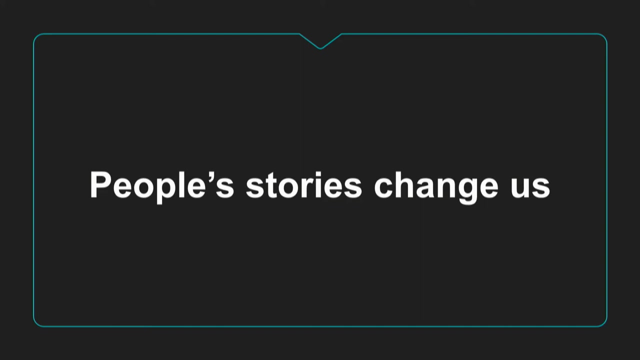 What I realized, though, is the film was just this manifestation of a simple, powerful idea. People's stories change us Right. Cody's story changed me. It literally Set the course for the next 14 years of my life. It's still a guy for me today. 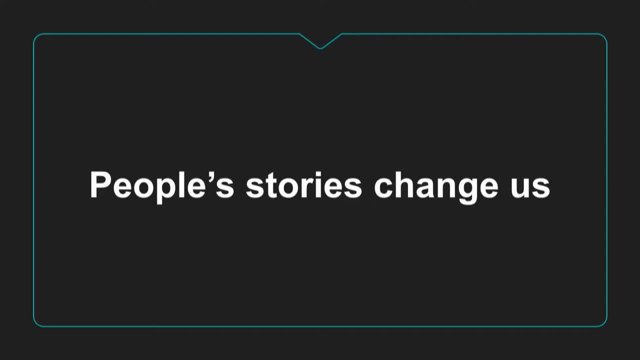 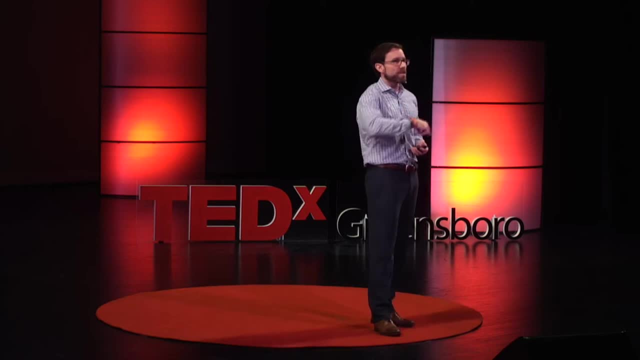 It's why I'm standing on this red dot right now, and it convinced for me not to give up on the broken system right, But to double down on the thing that I think matters most to all of us here today, Which is to know that we exist, to know that we belong and to know that our lives matter. 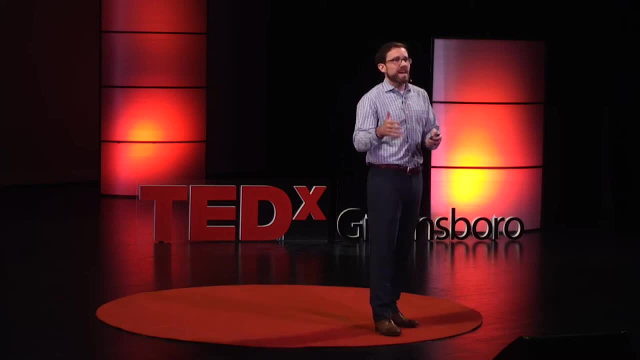 and so Right after Cody ages out, He decides he's going on this mission. He's gonna go on this mission to find his dad, a man He had never met before in his life. So he finds his dad in Phoenix Arizona. He goes down to visit him, spends two weeks, comes back. 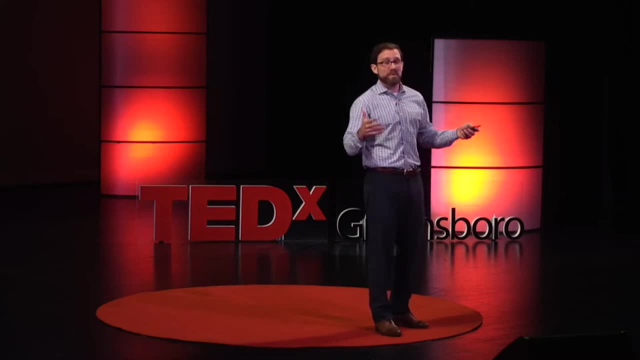 I meet him at the bus station and I Ask him, Cody, What was it like to meet your dad? And his answer was just one simple sentence, four words. it was pure joy, Joy, okay. So I asked him, Cody, why was it pure joy? 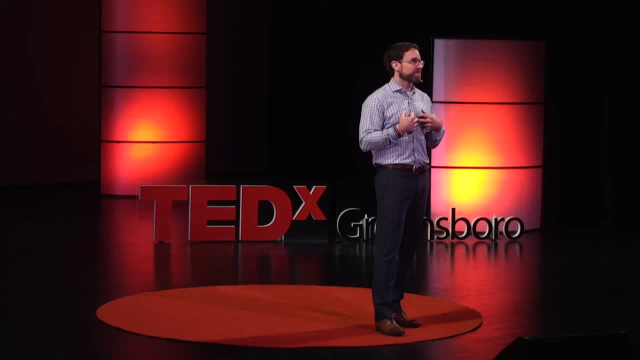 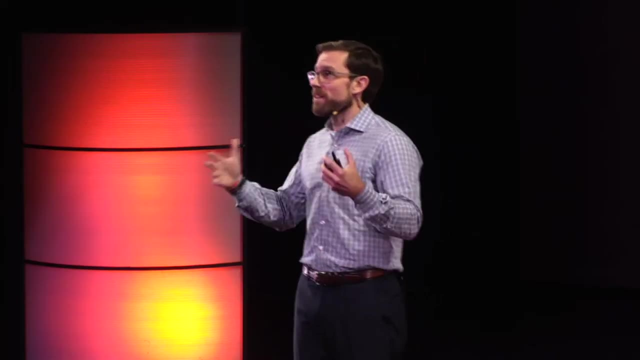 And he said to me: you know, I know what my dad looks like and he looks like me, and I know what my dad acts like and he acts like me. and He taught me all these things: how to clean the car, how to make pancakes, right, all these little things. and I'm thinking again. 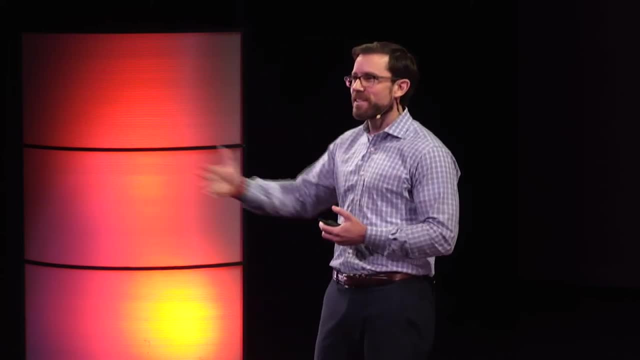 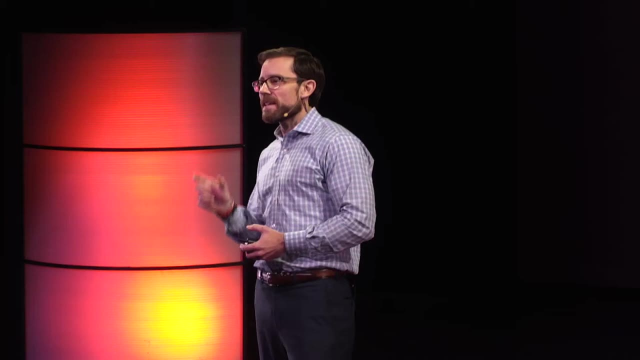 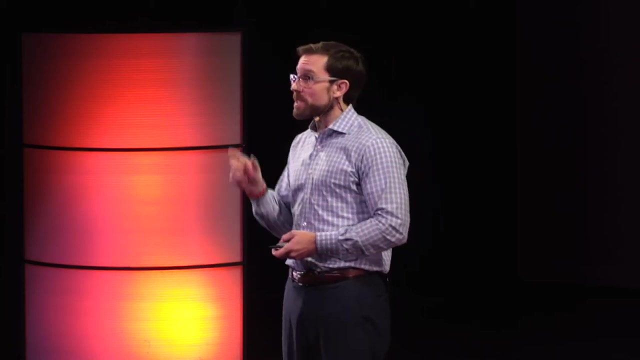 in the back of my mind, Cody, these are all the things I tried to teach you, and you had no time for it when you were in foster care, And then I realized eventually that it was the relationship with his dad that made all the difference. right, Cody's story taught me that our job is to 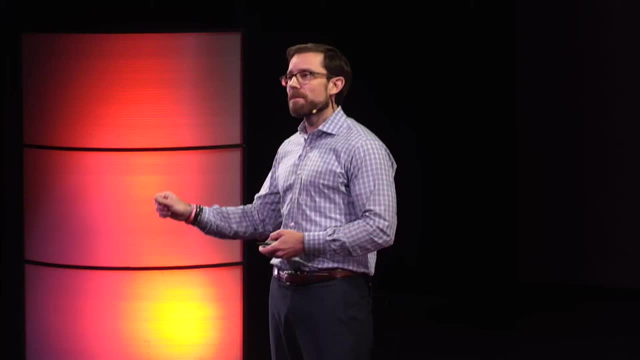 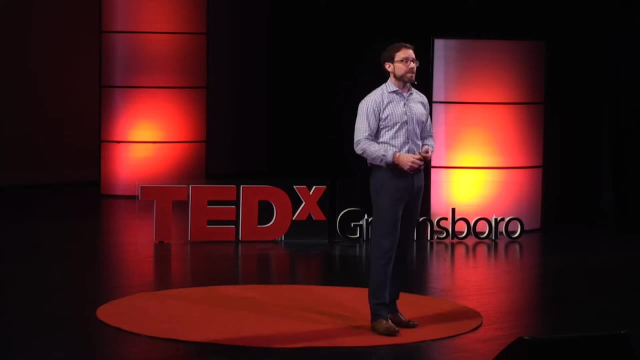 prioritize relationships to put family first. So I spent my career trying to improve the foster care system to prevent kids from aging out of foster care by putting family first, And we've achieved a lot of successes. So you know we have scaled programs that prevent hundreds of kids. from aging out of foster care in North Carolina. We've changed policies that have improved the experience of the foster care system for tens of thousands of kids in North Carolina. We've literally moved millions of dollars into the system to make it better. And here we are with 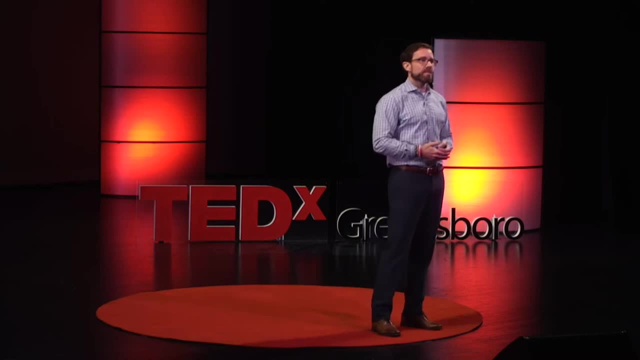 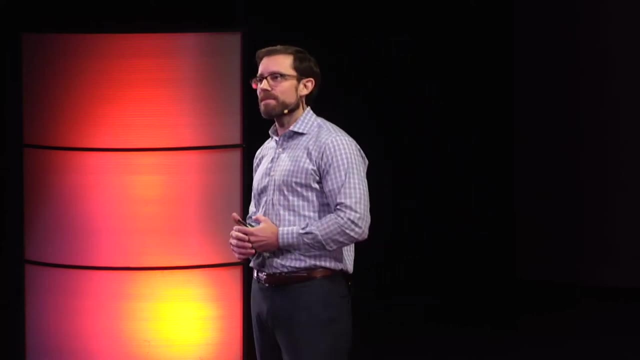 more kids in foster care today than when we started working on those initiatives. So even more recently, I started talking to my dad about how I wanted to improve the foster care system And he said: I'm talking to more parents who have experienced the child welfare system, listening to their 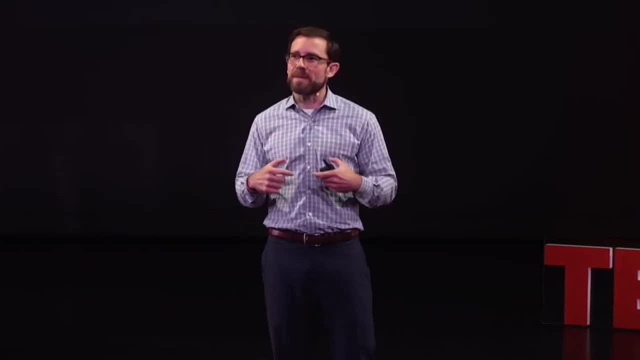 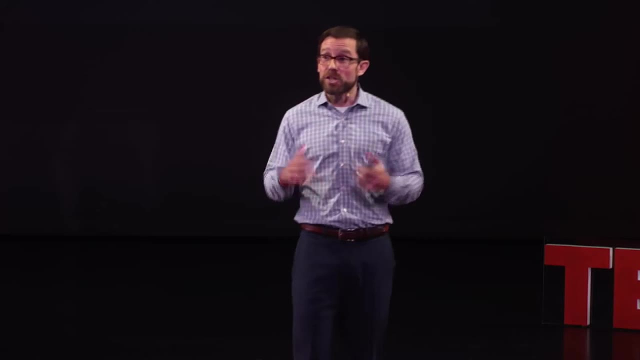 stories, learning from their experiences. And their stories have changed me. Their stories have given me a new perspective. right that our job is not to improve the foster care system, Our job is to transform it. right. Our job is to keep families together and to prevent foster care in the first. 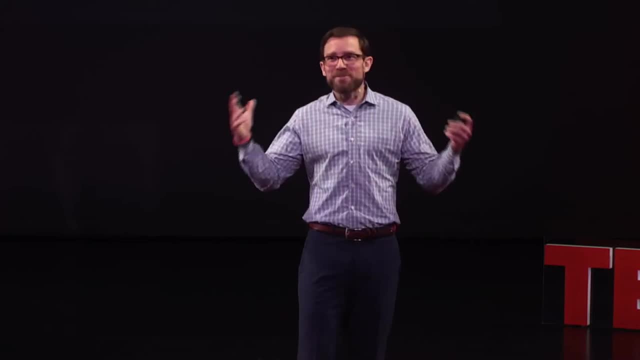 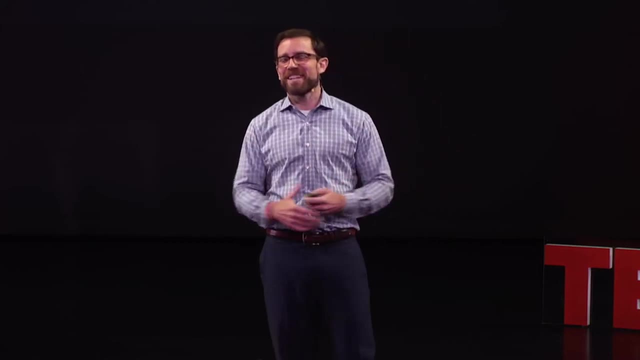 place. So how do we transform America's child welfare system so that families can thrive? It's a big question. No real clear, straightforward answers to it, But I think there's a place that we can start. Change starts with us. We change through people's stories. We start by listening. 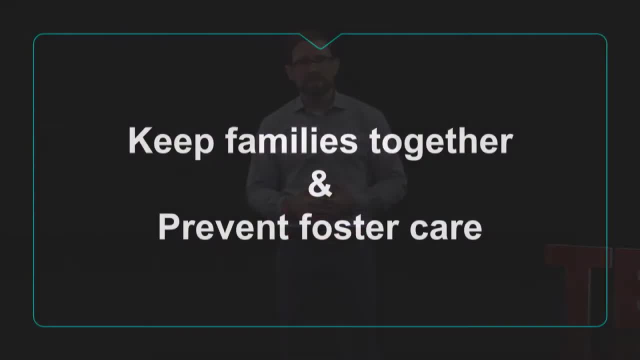 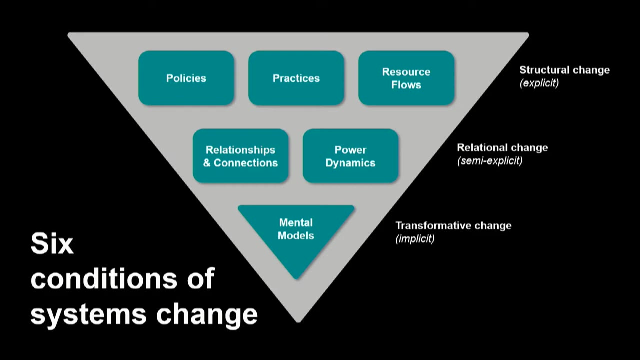 right, We listen to people's stories And when we change, we change through their stories. When we change, we change the system. But stories are not enough. right, There are six things that we need to change, Six conditions of systems change, Structural changes. right, The first three, Three that I just 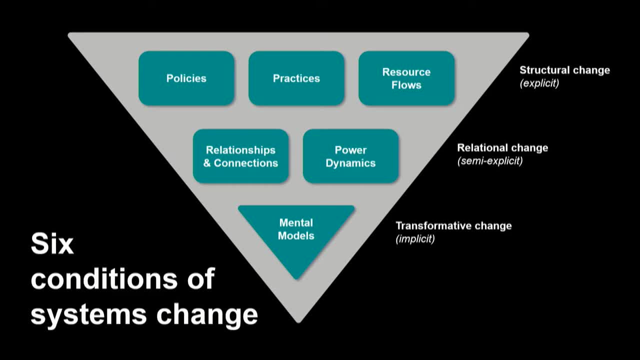 talked about Policy practice, changing the flow of money. right, These are necessary, important changes, but not the place that we start right. We have to ask ourselves, before we make those changes, who has the power to make decisions about those changes? Who ultimately benefits? 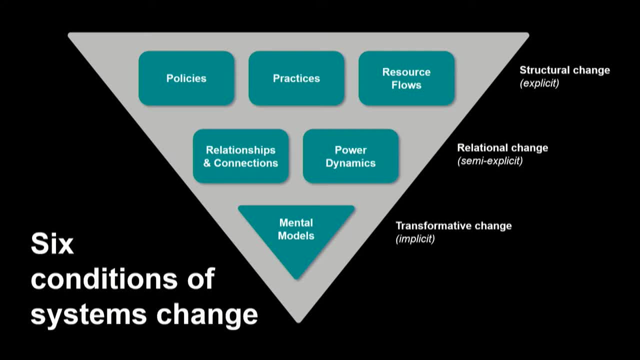 from those decisions right. So that takes us to the next two: right Relationships and power dynamics. We have to bring the right people together. right, We have to bring a different people to the table. We have to bring a diverse set of perspectives. We have to bring together people. 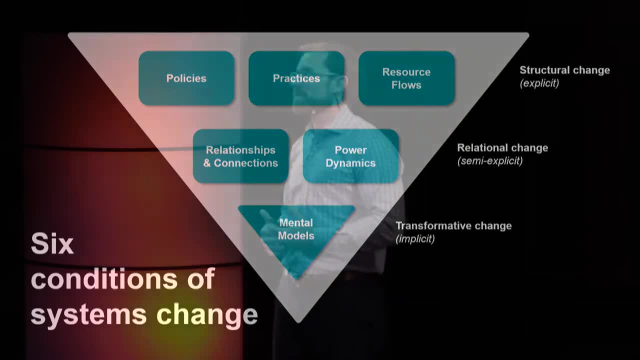 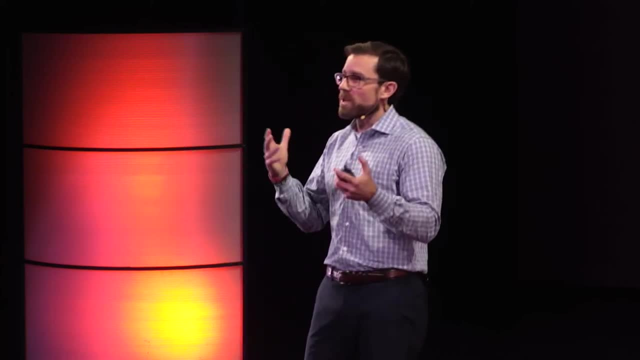 that have lived the experience of the child welfare system right. We have to create this inclusive table. That's the secret sauce, I think, of systems change. It's the place that we can build relationships, We can build trust And from that foundation we can shift power right Shift. 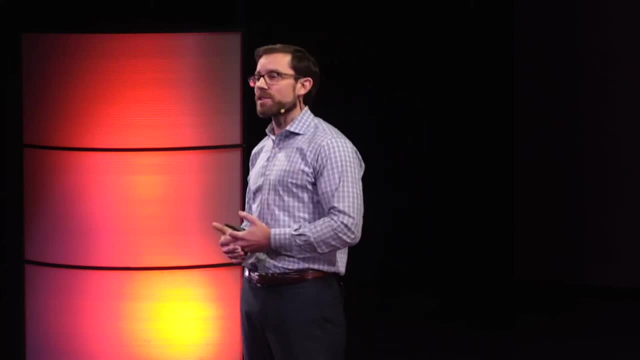 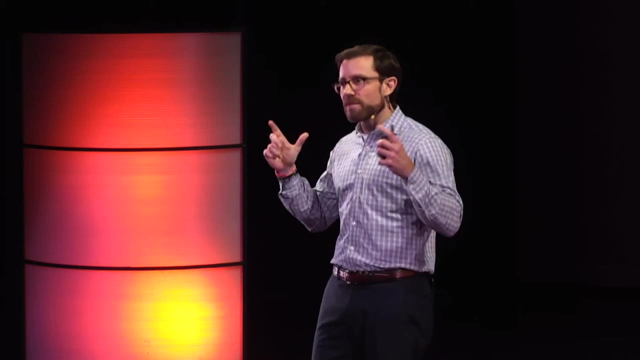 power to people that have lived the experience of the system to inform decisions that we might make about structural changes. But before we can do that we have to shift mental models right. That's hard work to do. We have to shift our mindsets first. right, So our mindsets are just our. 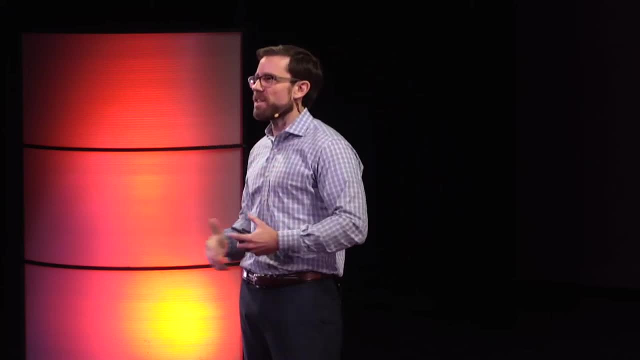 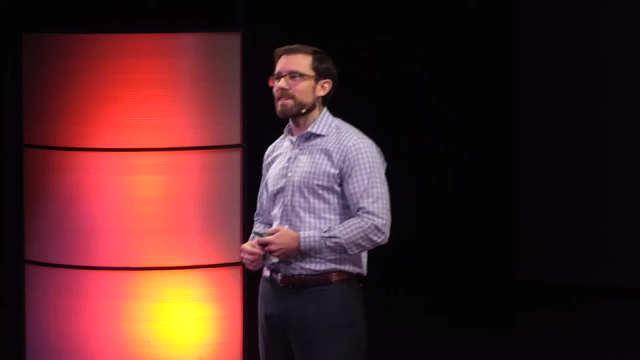 deeply held beliefs, our patterns of thought. These are our behaviors, our decisions, right? So how do we shift our mindsets? That's where I think the power of story becomes so important. right, We listen to somebody's story. We put ourselves in somebody else's shoes. right, It gives us a 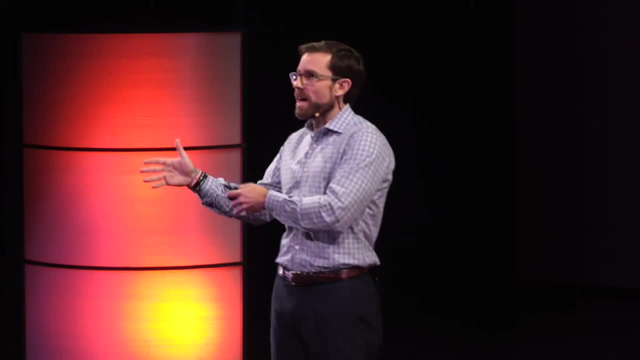 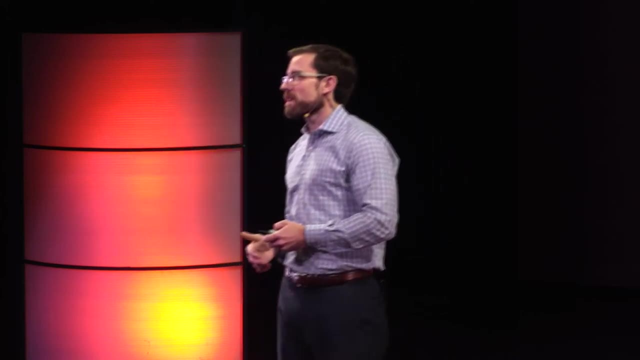 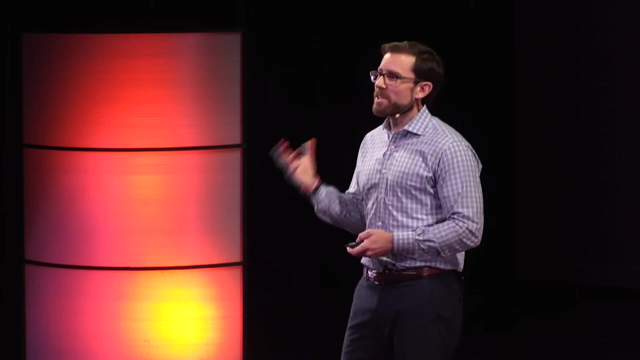 different perspective about how to see the world right And that has the power to shift our mindset right, To maybe create that inclusive table, go a different direction around structural changes. So we start with stories. So let me give you an example of this. So when we started making the film, I asked all the young people in the film 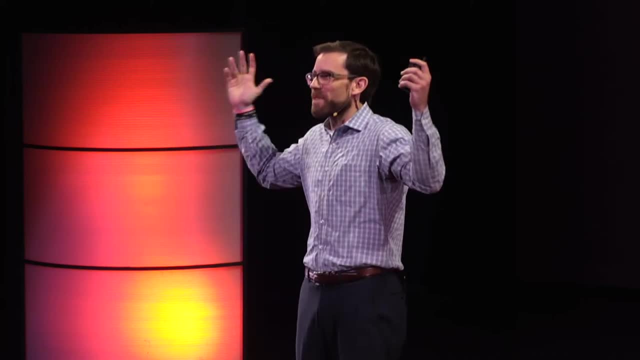 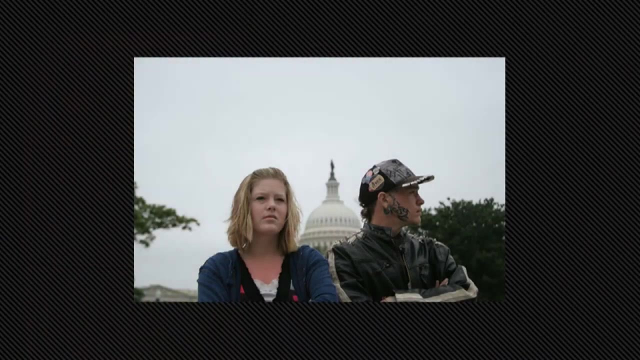 why do you want to share your story, Like, why would you want to put your life on the big screen, right? It's very personal stuff. And so they all had two answers in common. One they said: you know, nobody ever asked me what it was like to be in foster care. 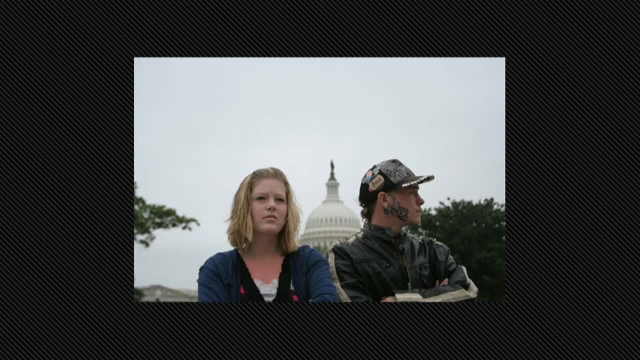 Two, they just wanted to know that their lives mattered, right. And then they said: you know, I want to share my story with people in a position of power to make the system better for the next generation. So this was our true north. And so we started asking ourselves: okay, so when you're a 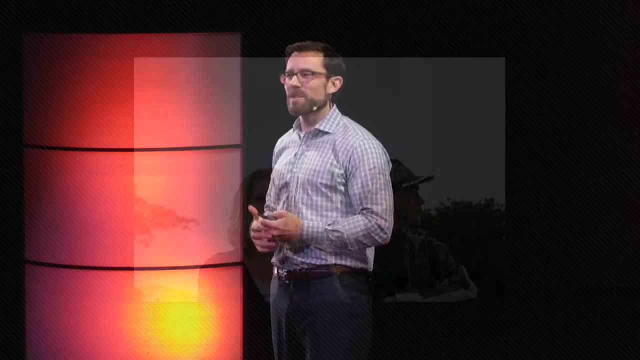 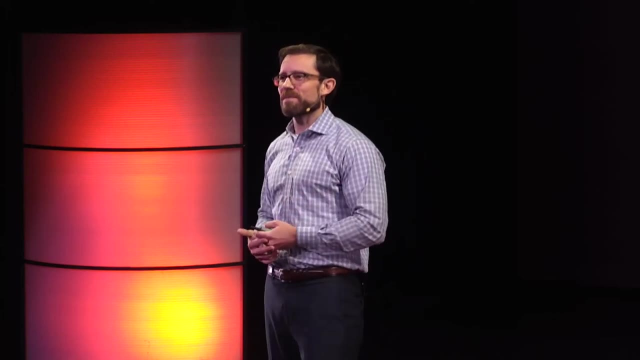 kid, who has all the power? right? Your parents, right? You remember when we butted heads with our parents as teenagers? Parents have all the power. So, if you're a kid in foster care, who are your parents? right? The government is your parents, ultimately. So we thought, okay, we should. 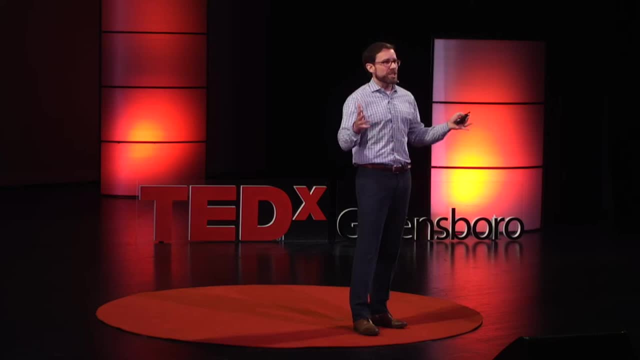 share our story. And so we did. And so we started asking ourselves, okay, who has all the power? And we, we talk to the government. And so this woman, Becky Shipp, was working on Capitol Hill and she was a staff to the Senate Caucus on Foster Youth and she invited Mandy and Rafe, two of the young people. 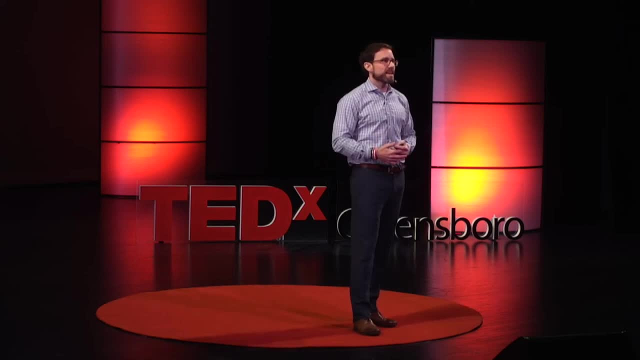 in the film- to come to Capitol Hill to testify, to share their testimony to the Senate Caucus on Foster Youth. And so they did and we go and we film it and they share their story and it's compelling and raw and authentic and they provide really deep insight, things that folks didn't know. 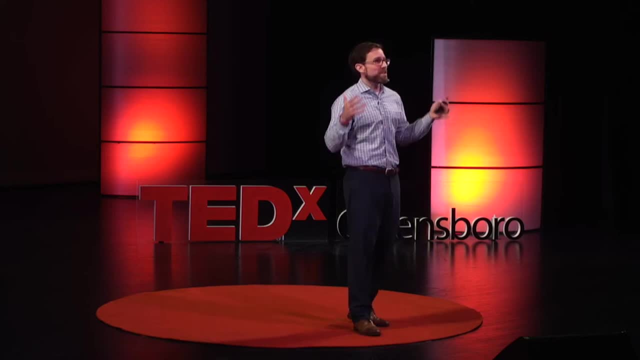 on the Hill. And so Mandy at one point in her testimony says: you know, if I don't have a family, who's going to teach me about dating or the prom? She said, who's going to walk me down the aisle? 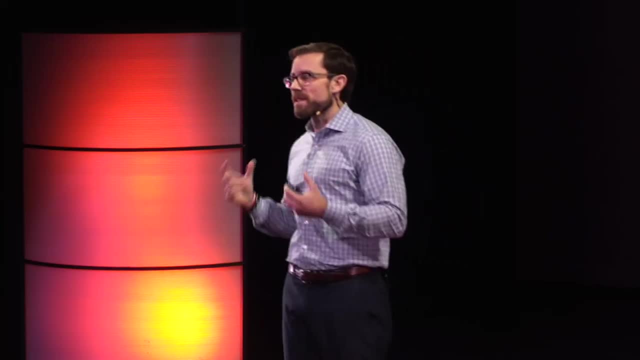 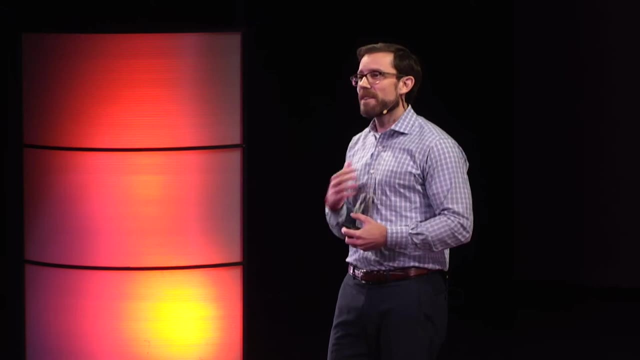 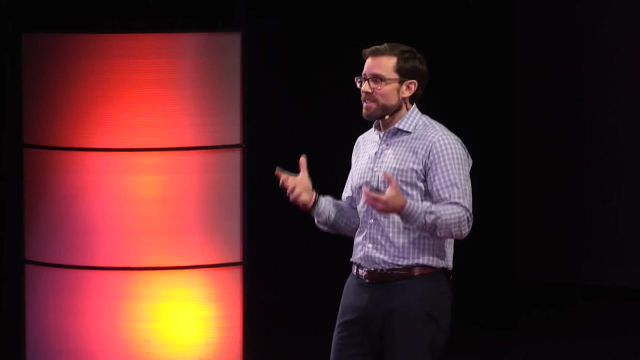 one day. And then Rafe said something that still gets me today. He said: you know, I may look tough, I may have this big tattoo on the side of my face, but I have a heart that would swallow everybody in this room. And he does, And they, they. 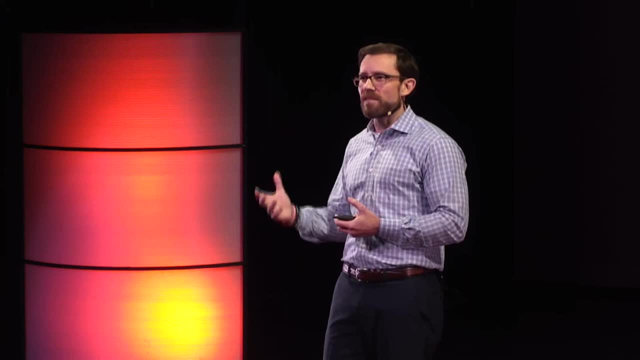 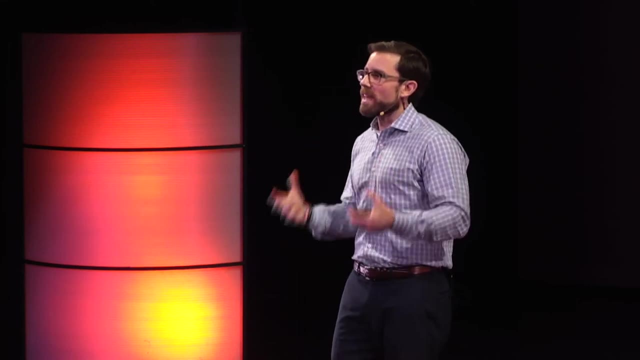 they shared their story that day and I think what they did was they challenged all of us to see beyond the surface right, to see beyond the face tattoo, to connect with them on this much more deeper human level, to put ourselves in their shoes, see the world from their perspective. 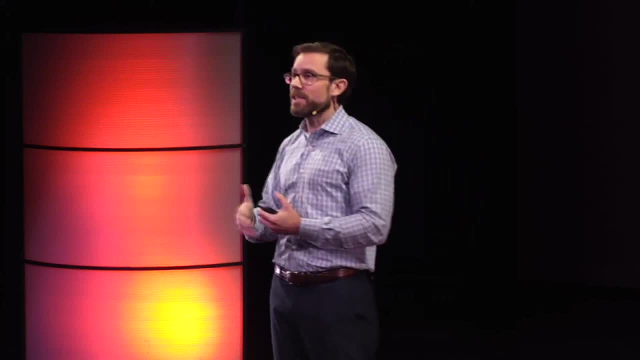 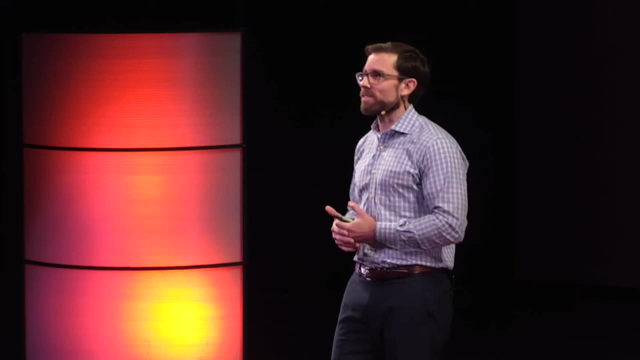 right, and that shifts mindsets. It shifted Becky's mindset. It changed her behaviors from that day. So what she did was she organized this series of six listening sessions and she brought young people from all over the country to Capitol Hill to share their story, share their. 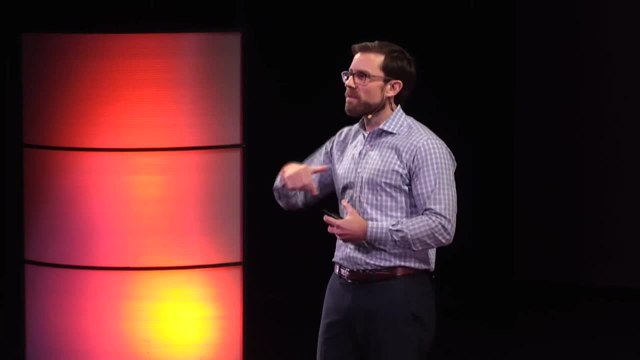 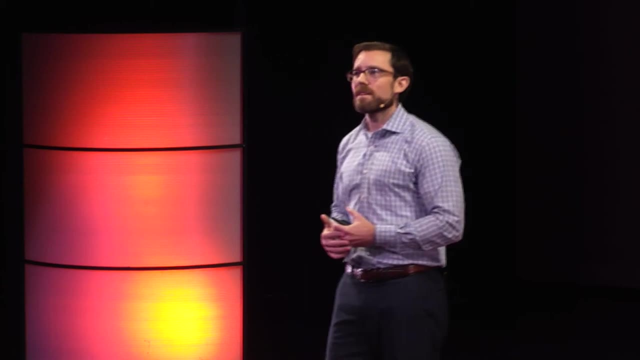 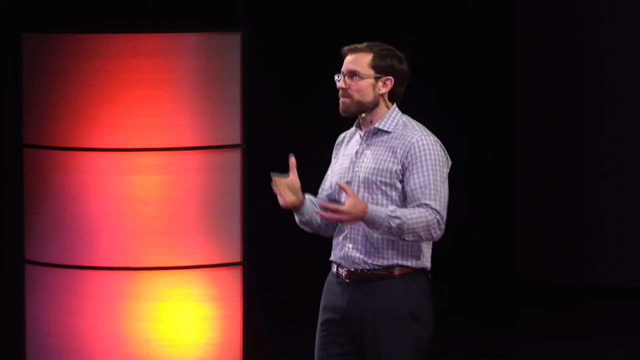 experiences, their ideas, their, their critiques of the system, and it was the content of those conversations that led to what became the Family First Act. right So, the Family First Act is one of the most significant pieces of child welfare legislation in in decades. It has the potential. 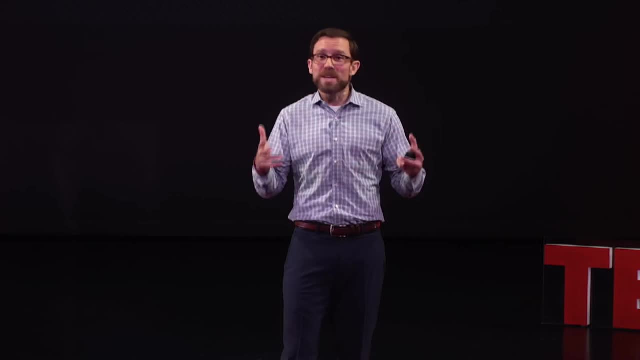 to be transformative. Now we'll see what happens. It's literally being implemented today. October 1st was a go-live date for it, so we'll, we'll see. But I think what's really really interesting about that is the process rather than the structural change right. The 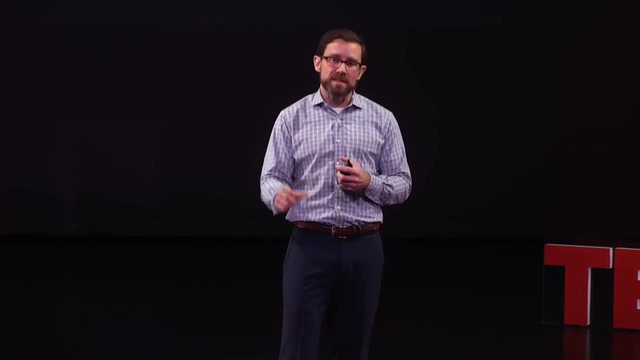 process started with somebody sharing their story, with somebody listening right Becky's shifting her mindset, changing her behavior, creating this inclusive table, right building relationships, and it was that, then, that led to the structural change. So I think that's where we need to. we 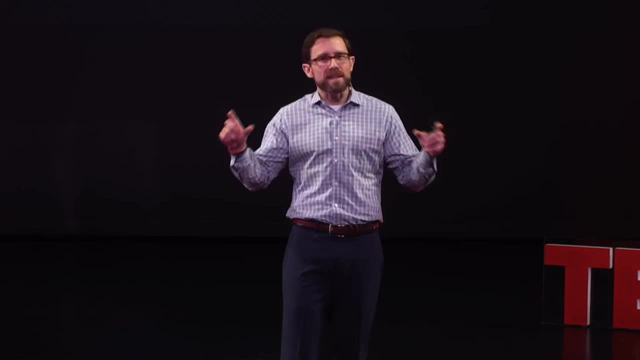 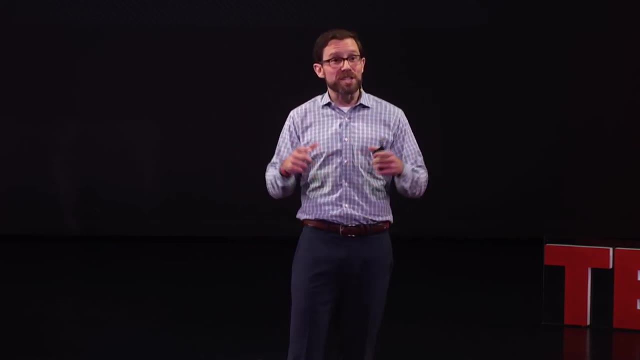 need to start again with story. We can replicate that process, but this time, instead of asking this question- how do we prevent kids from changing their story? We can replicate that process, but we can't prevent kids from aging out of foster care. We ask the question: how do we prevent? 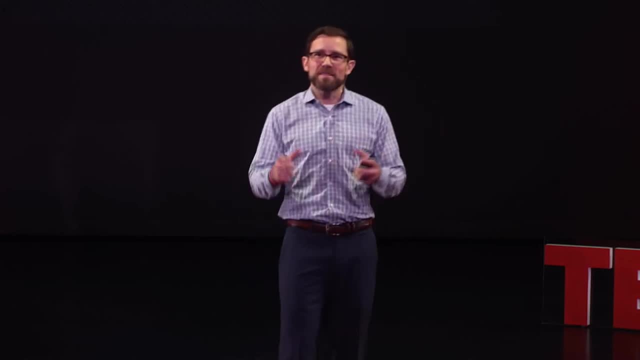 foster care in the first place, And we ask parents and families and communities that question right, And so when we do that, I think what we'll find is that there are opportunities. So one of the things that we know is that families come to the attention of the child. welfare system for neglect far more often than they do for abuse, physical abuse, physical harm to children. 60% of all child protective service responses are for neglect only right, not for physical abuse or harm, which we most often think about. So what is neglect, Neglect? 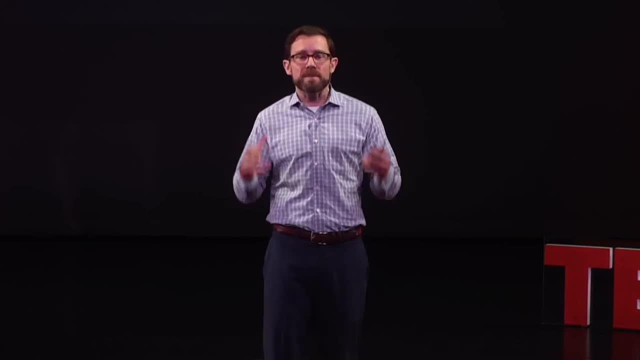 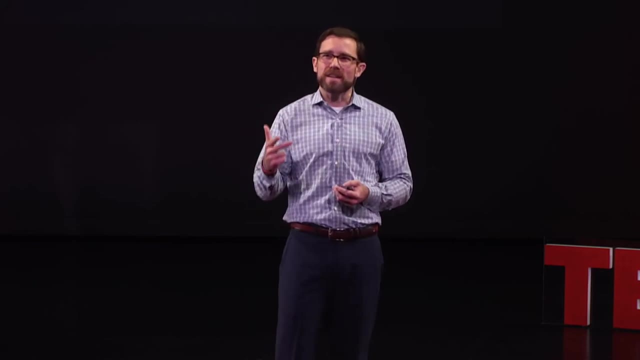 really looks like the overburdened parent, the overburdened family families dealing with difficult, stressful, largely systemic conditions. right Things like access to health care or child care or safe housing, access to mental health services or substance use services- right. 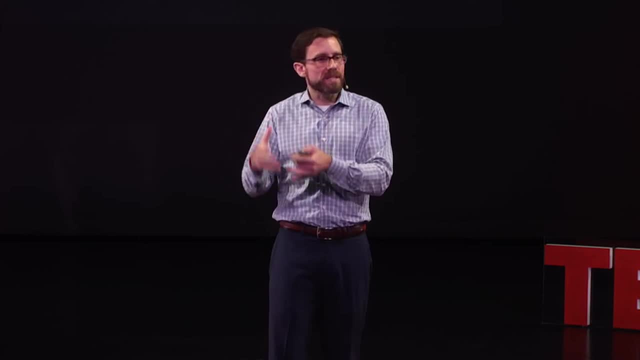 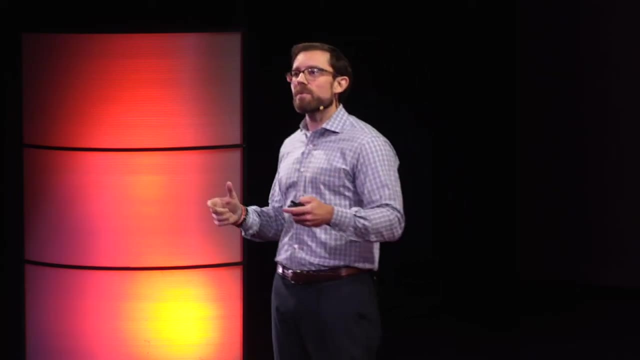 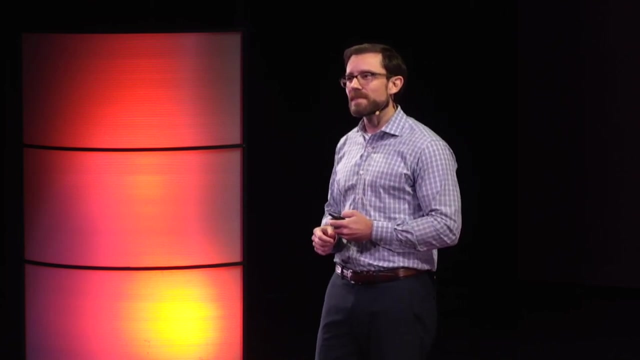 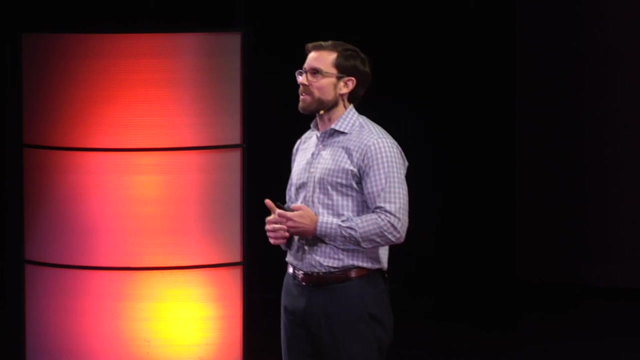 this is often more about these difficult, stressful conditions than it is about bad parenting or bad parenting behaviors, And so another thing that we know is that family income is one of the greatest predictors of child welfare involvement. So when states decrease economic investments to support families, we tend to see an increase in child welfare. 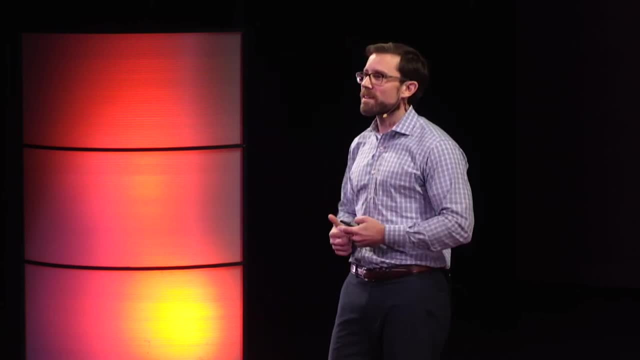 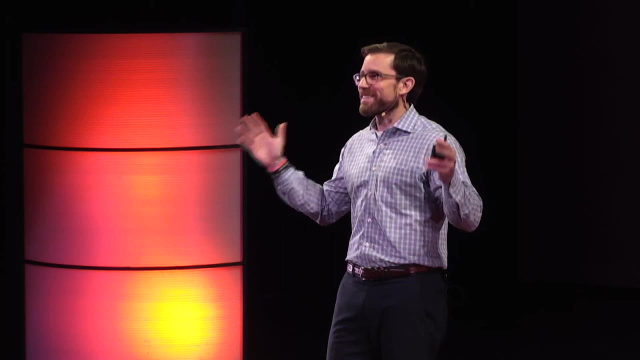 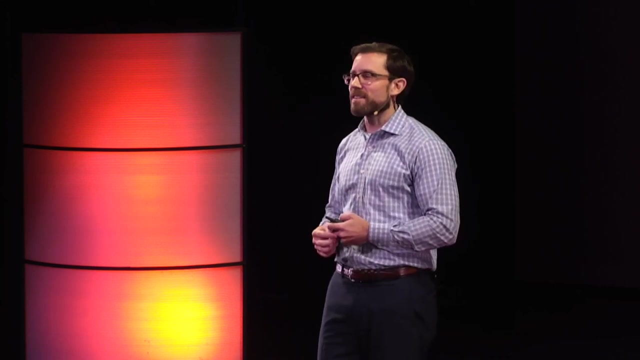 involvement And when states increase investments to support families, we tend to see child welfare involvement decrease. So that's a pretty broad, blanket statement, clearly. But there is a longstanding body of research that shows us this association And, for example, a $1 increase in the minimum wage is associated with a 9 to 10% decrease in child maltreatment. Yet we aren't prioritizing family and family well-being with our investments. In fact, in 2018, we spent $33 billion on child welfare expenditures. This is largely spent on foster care, And of that, $33 billion, less than 15% was spent on activities that would prevent the need for foster care. So how do we flip that percentage or at least start to shift our priorities, our resources, our investments, upstream, upfront, to support families, to keep families together, Do we? have to accept that there are 700,000, 000 families out there that need to share with families? Or do we have to accept that there are 700,000, 000 families out there that need kids separated from their families in foster care every single year? 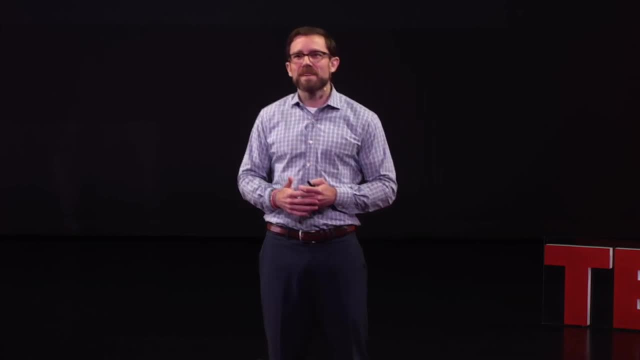 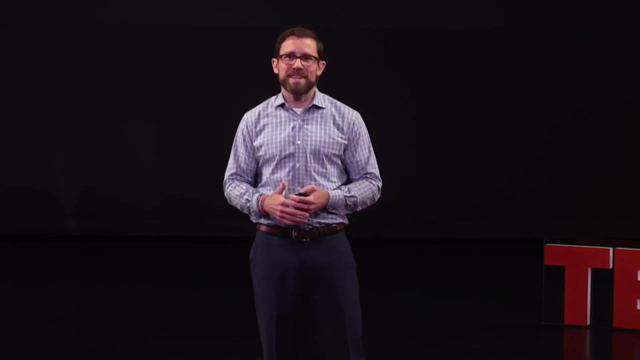 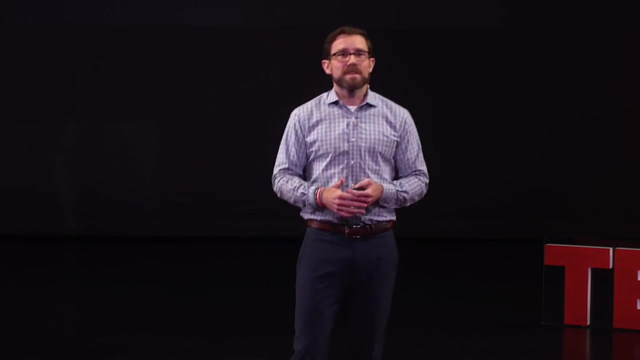 So I want to end with just a few thoughts. First, you know our care and concern for the safety of children is undoubtedly important and it always will be When we have to keep kids safe. we need ways to keep kids safe, But what I would suggest is we can demonstrate our care and concern. 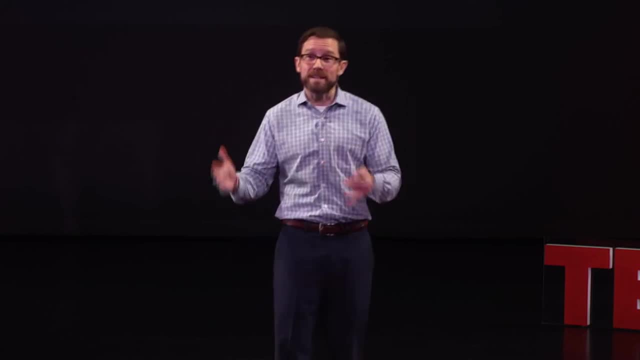 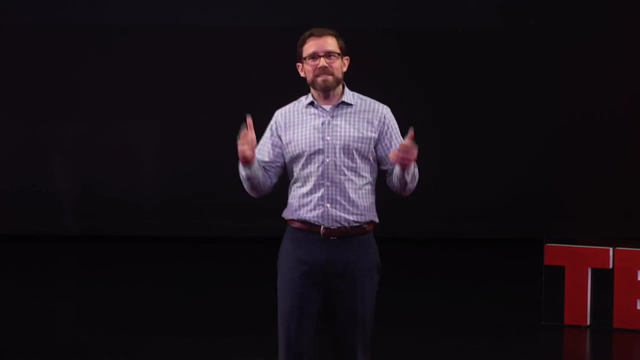 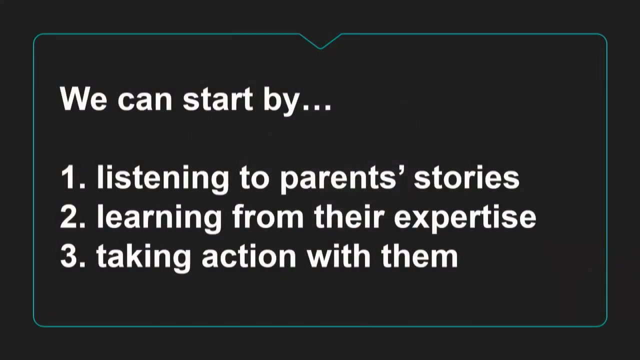 for children by investing in the well-being of their parents. And we can start today. simply, We can ask parents what they need right, Listen to their stories, We can learn from their experiences, from their expertise, We can create that inclusive table right And we can find ways.